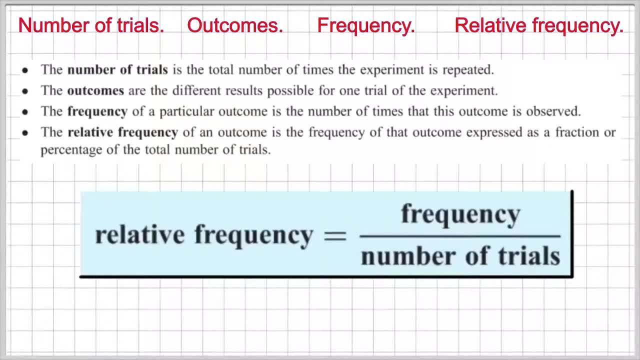 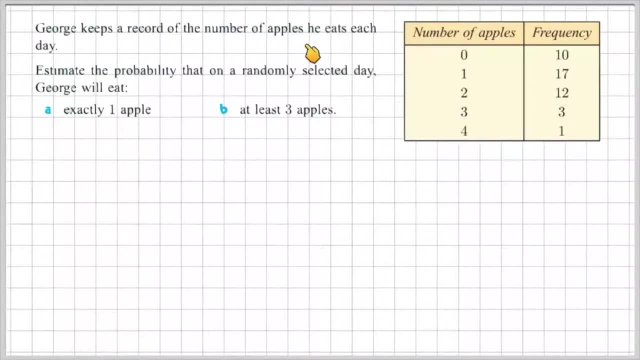 relative frequency, which is the frequency over the total number of trials. Okay, so let's do an example using relative frequency. So George keeps a record of the number of apples he eats each day. Estimate the probability on a randomly selected day that George will eat exactly one apple and be 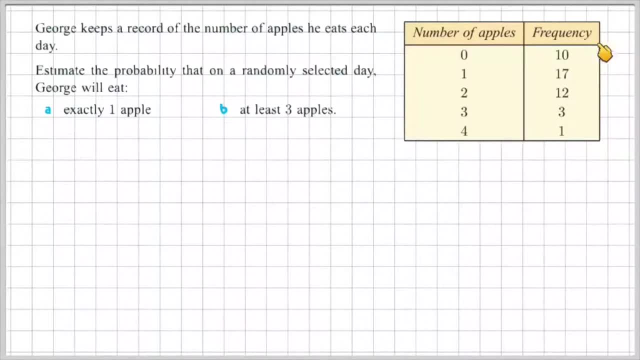 at least three apples. So we're going to be using this table of values to answer the question. We can see from the table that George has recorded data for 43 days, and that is 10 plus 17 plus 12 plus 3 plus 1 days altogether. 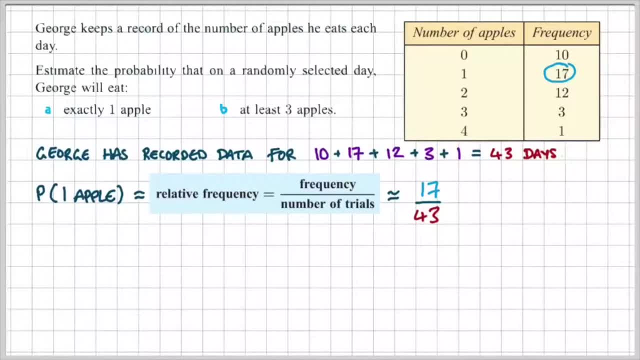 Now, in order to find the probability that George is going to eat exactly one apple, we're going to use relative frequency, That's the frequency divided by the number of trials. So we know from the table that George ate exactly one apple on 17 different days. 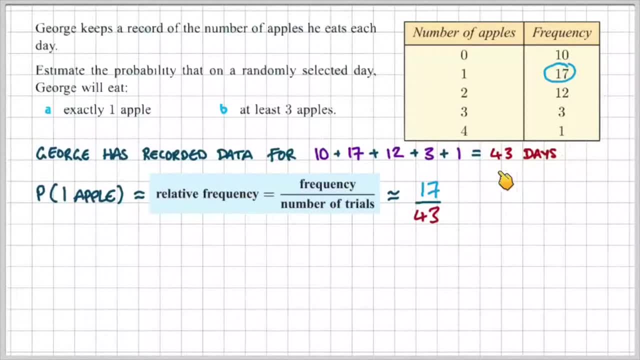 So that will be 17 divided by the number of trials, which is 43 days. So 17 divided by 43 will give us an approximate value of 0.395.. Or we could say that the probability of George eating exactly one apple is about 40% of the time. 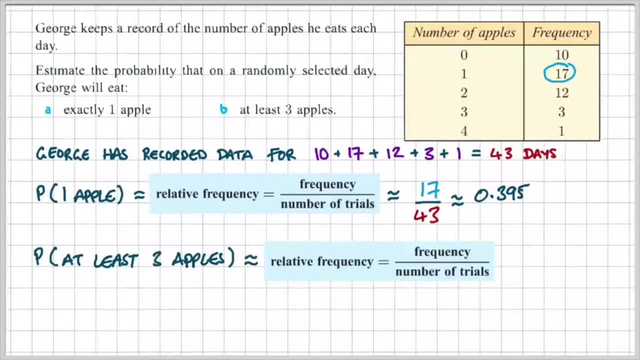 Okay, part B: The probability that George eats at least three apples. So the word at least here can refer to the fact that George could eat three or more apples. So in this case he can eat three or four apples, because that's the data that we have in the table. 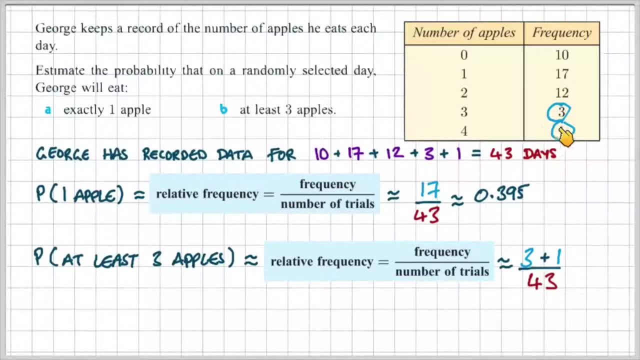 So from the table we can see that George eats three apples three days and four apples on one day. So in total we can say that's 3 plus 1, which makes 4 over 43, which gives us a probability of 0.3. 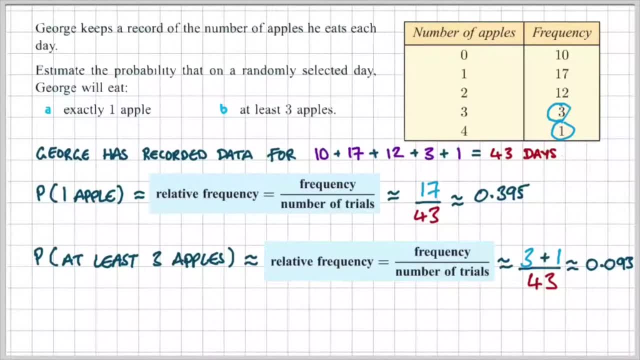 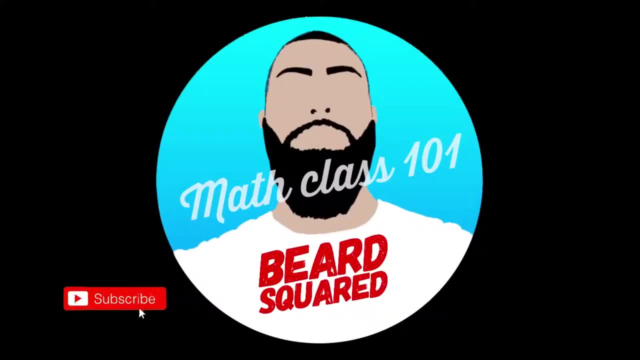 So that's 0.093, or about 9% of the time. George is going to eat at least three apples. Okay, let's look at a different example where we have group data. This table shows how long Nathan has slept each night recently. 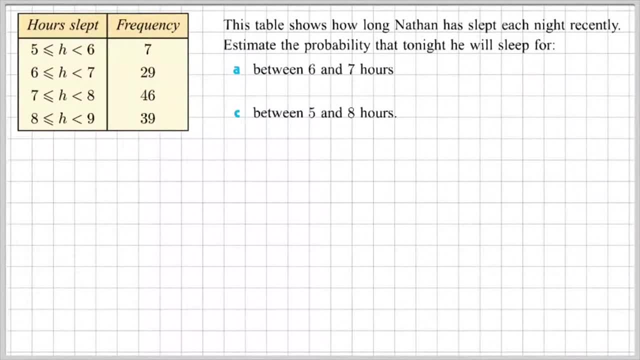 Estimate the probability that tonight he will sleep for A between 67 hours and C between 5 and 8 hours. So pause the video here, see if you can do this for yourself, and then play when you're ready And I'll show you.